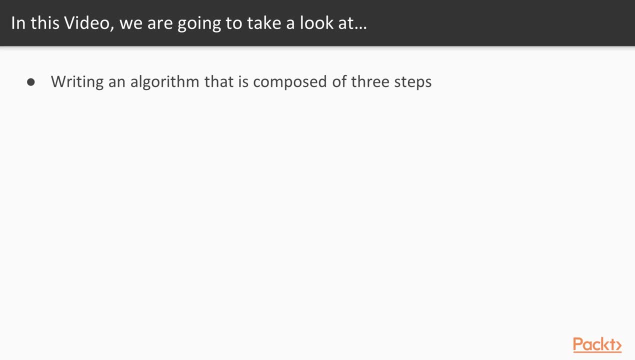 steps are controlled by the template, and just the second step is deferred to the user. The template pattern is one of those widely used patterns that are incredibly useful, especially when writing libraries and frameworks. The idea is to provide a user some way to execute code within an algorithm. 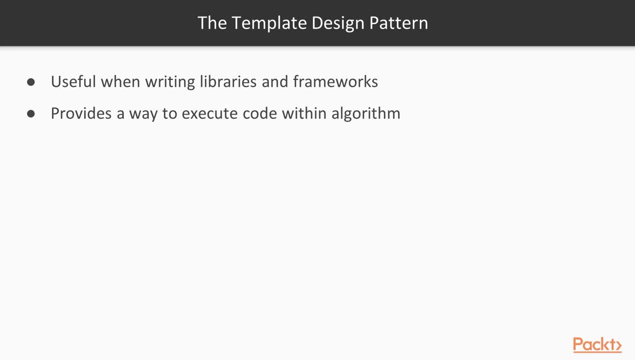 In this section we will see how to write idiomatic Go template patterns and see some Go source code where it's wisely used. We will write an algorithm of three steps where the second step is delegated to the user, while the first and third aren't The first. 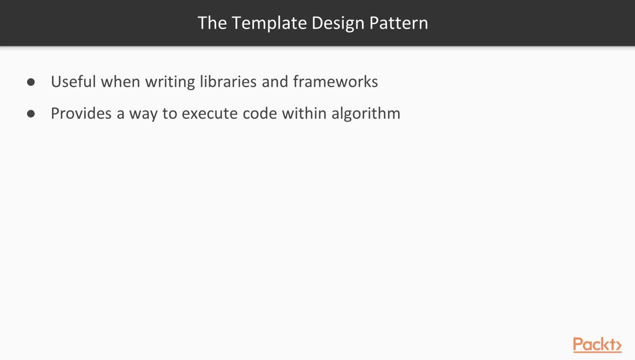 and third steps of the algorithm represent the template. While with the Strategy Pattern we were encapsulating algorithm implementation in different strategies, with the Template Pattern we will try to achieve something similar, but with just part of the algorithm. The template design pattern lets the user write a part of. 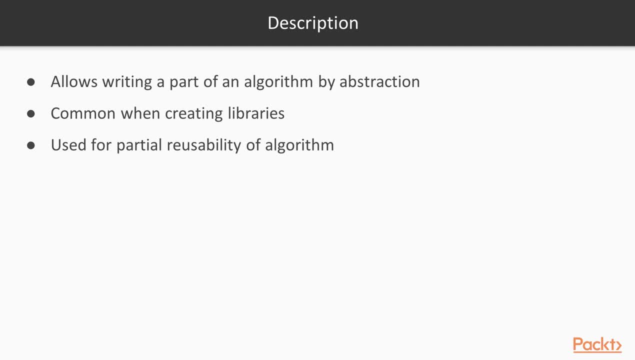 an algorithm, while the rest is executed by the abstraction. This is common when creating libraries to ease in some complex task or when reusability of some algorithm is compromised by only a part of it. Imagine, for example, that we have a long transaction of HTTP requests We have to perform. 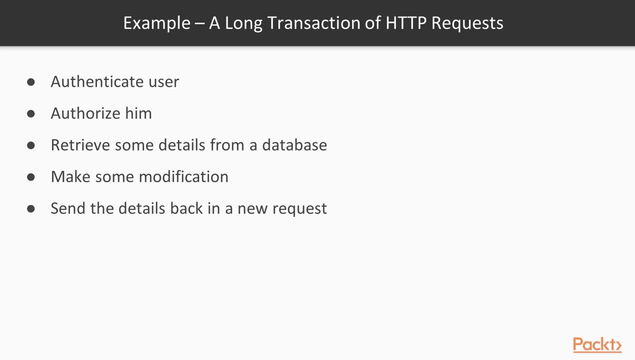 these steps. First, we authenticate user and then authorize him. Next, we retrieve some details from a database and make some modification. Lastly, we send the details back in a new request. It wouldn't make sense to repeat steps one to five in the user's code every time he needs to. 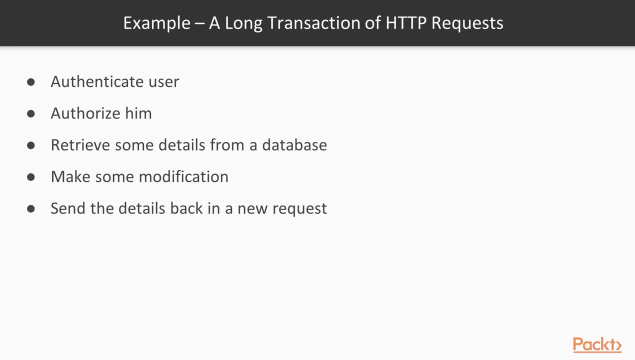 modify something on the database. Instead, steps one, two, three and five will be abstracted in the same algorithm that receives an interface with whatever the fifth step needs to finish the task. It doesn't need to be an interface either. It could be a callback. The template design pattern. 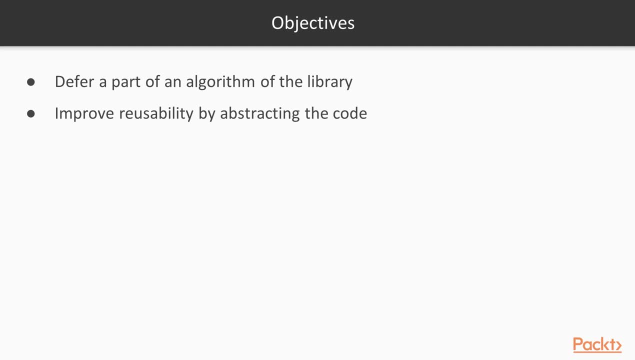 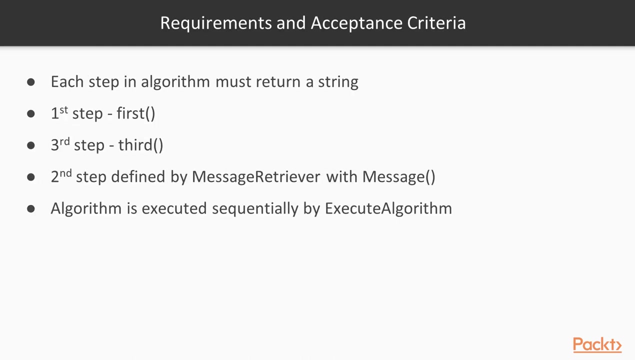 is all about reusability and giving responsibilities to the user. So the objectives for this pattern are listed here: Defer a part of the algorithm of the library to the user and improve reusability by abstracting the parts of the code that are not common between executions. A brief description of 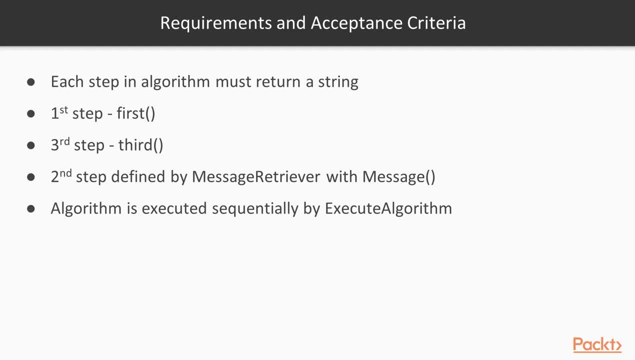 what the template pattern has to do is to define a template for an algorithm of three steps That defers the implementation of the second step to the user. Here are the requirements and acceptance criteria for our example. So each step in the algorithm must return a string and the 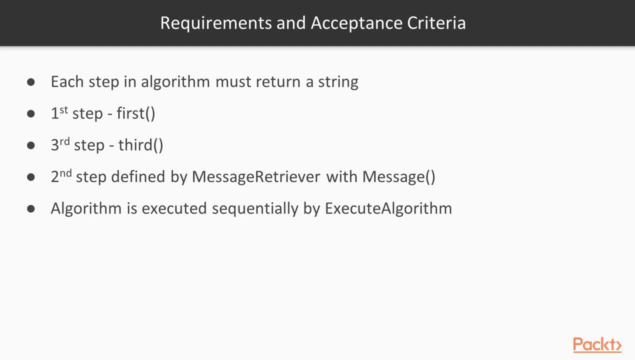 first step is a method called first and returns the string hello, While the third step is a method called third and returns the string template. Then the second step is whatever string the user wants to return, but it's defined by the message retriever interface that has a message string. 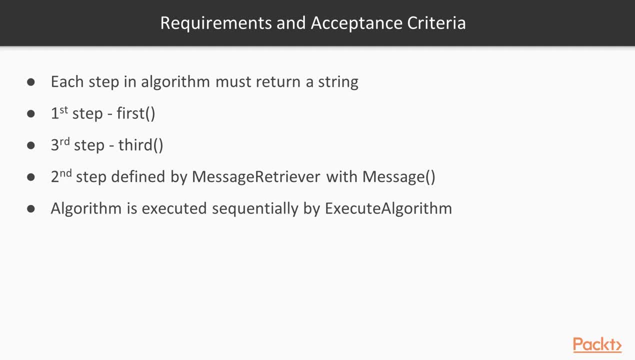 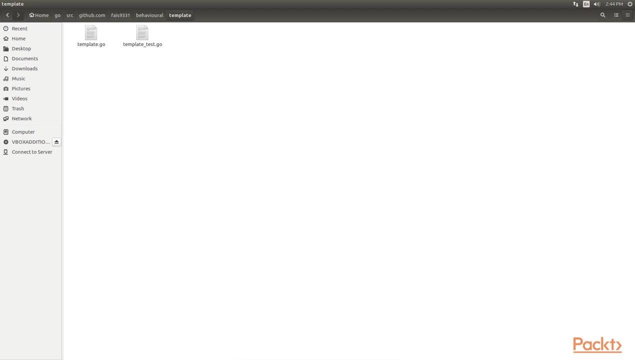 method. Finally, the algorithm is executed sequentially by a method called execute algorithm and returns the strings returned by each step, joined in a single string by a space. Now let's move on to the unit tests for the simple algorithm. Now we will focus on testing the public methods. 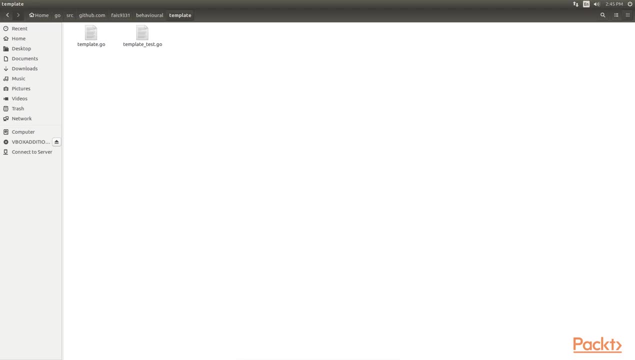 only. This is a very common approach. All in all, if your private methods aren't called from some level of the public ones, they aren't called at all. We need two interfaces here: One for the template implementers and one for the abstract step of the algorithm. 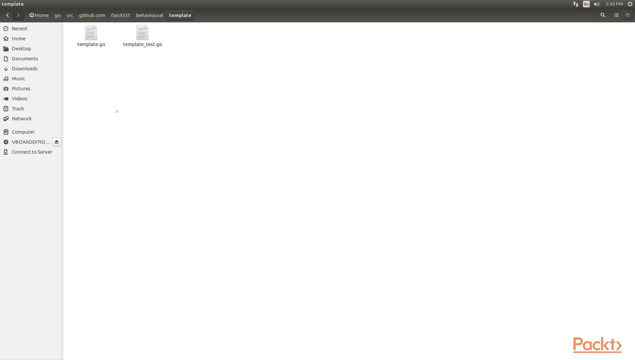 As you can see, I have created a folder called template and I have two files created here with the names templatego and template underscore testgo. So let's open templatego Here. let's add the package name and type interface. A template implementer will accept. 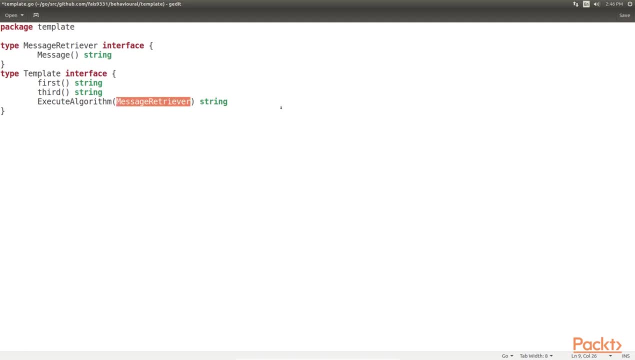 a message retriever interface to execute as part of its execution algorithm. We need a type that implements this interface called template. We will call it templateimpl. Let's add the code for the template implementer struct. So our first test checks the fourth and fifth acceptance criteria. 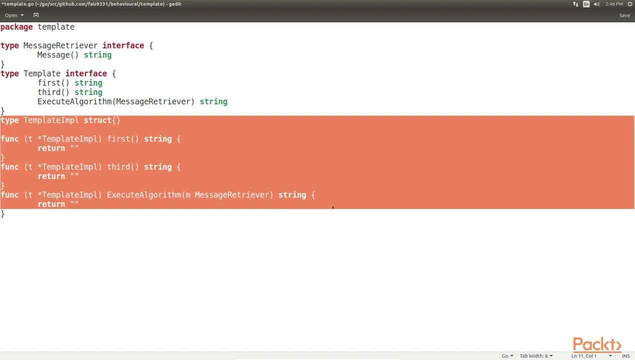 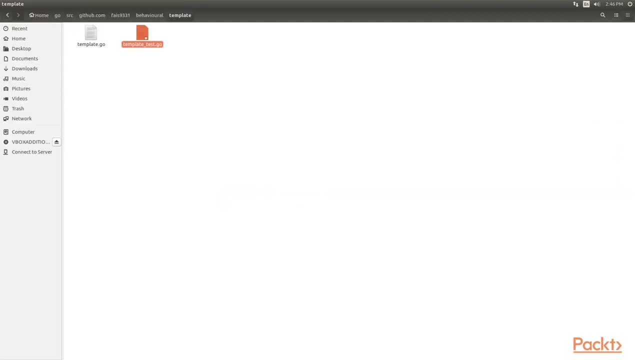 We will create the test struct type that implements the message retriever interface returning the string world, and has embedded the template so that it can call the execute algorithm method. It will act as the template and the abstraction. Let's save this. Let's save this file for now and move on to template testgo. Here we have named the package. 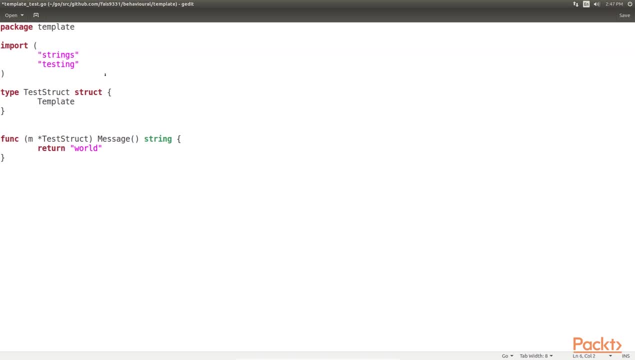 as template and imported strings and testing. Since this is a test, first define the test struct type. In this case, the part of the algorithm deferred to us is going to return the world text. This is the string we will look for later in the test doing a check of type. 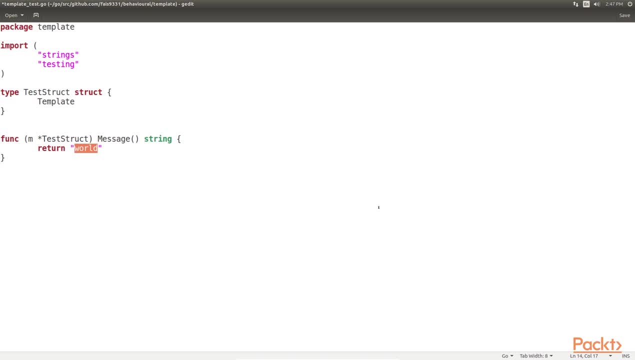 Is the word world present in this string? Take a close look. The test struct embeds a type called template. This is also the type we call the message retriever interface, which represents the template pattern of our algorithm. When we implement the message method, we are implicitly implementing: 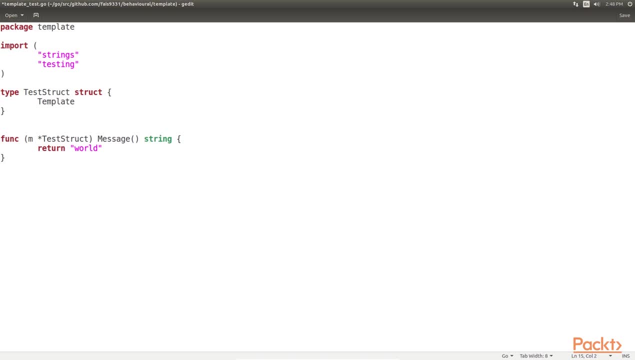 the message retriever interface. So now we can use test struct type as a pointer to a message retriever interface. Next let's add the code for the function test template algorithm. In the test. we will use the type we have just created When we call the execute algorithm. 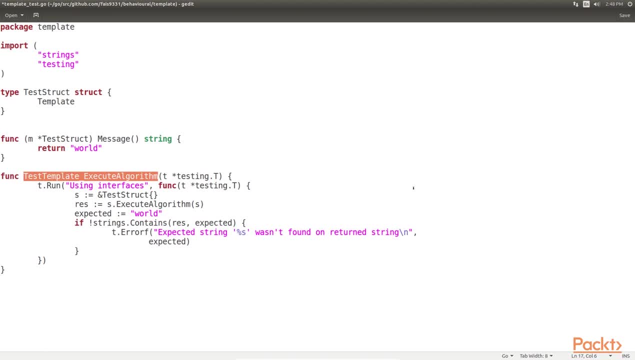 method we need to pass. the message retriever interface implements the message retriever interface. we can pass it as an argument, but this is not mandatory, of course. the result of the execute algorithm method as defined in the fifth acceptance criterion must return a string that. 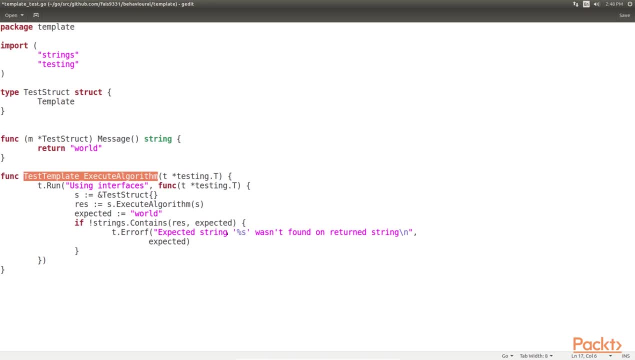 contains the returned value of the first method, the returned value of test struct, that is, the world string, and the return value of the third method, separated by a space. our implementation is on the second place. that's why we check that a space is prefixed and suffixed on the string world. so if the returned string 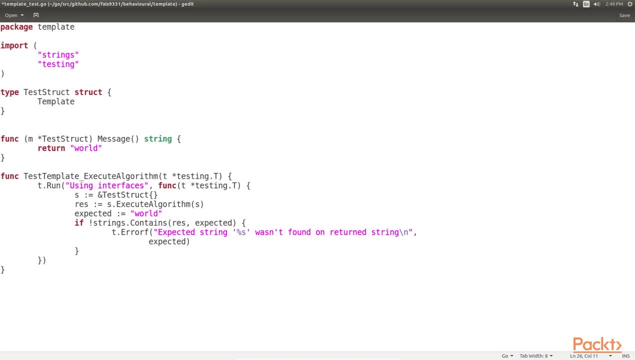 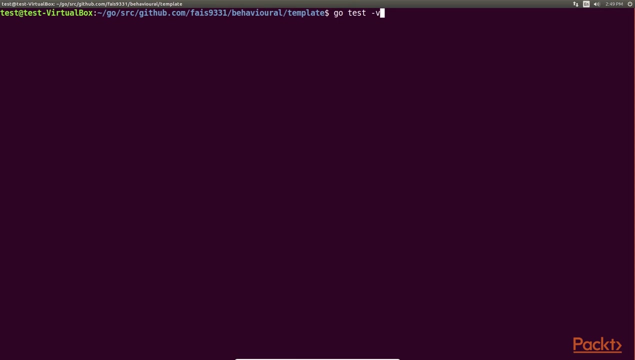 when calling the execute algorithm method doesn't contain the string world, the test fails. this is enough to make the project compile and run the tests that should fail. let's save this file and open the terminal type, the command go test hyphen V. as expected, the test fails. cool time to pass the. 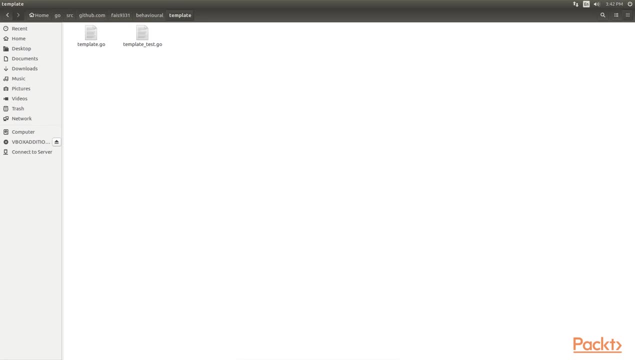 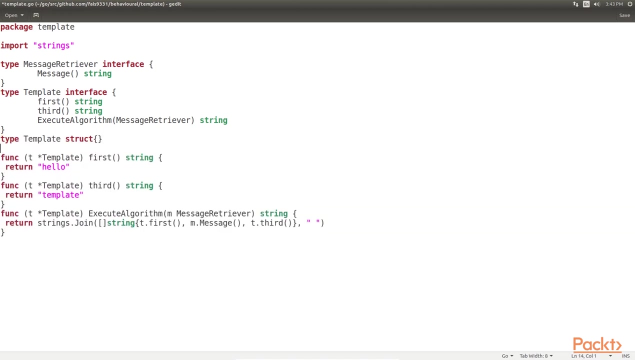 implementation of this pattern as defined in the acceptance criteria. we have to return the string hello in the first method and the string template in the third method. that's pretty easy to implement. open the template dot go file and let's modify the code here. let me add proper indentation. also, make sure to change the type template. 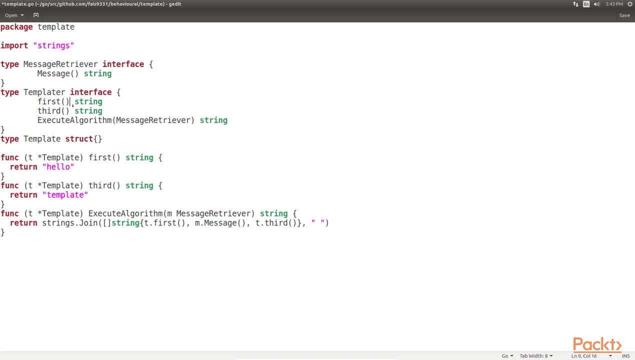 interface to template er, as we cannot have to type with the same name, save the file. we should be covering the second and third acceptance criteria and partially covering the first criterion, that is, each step in the algorithm must return a string. to cover the fifth acceptance criterion, we define an execute algorithm. 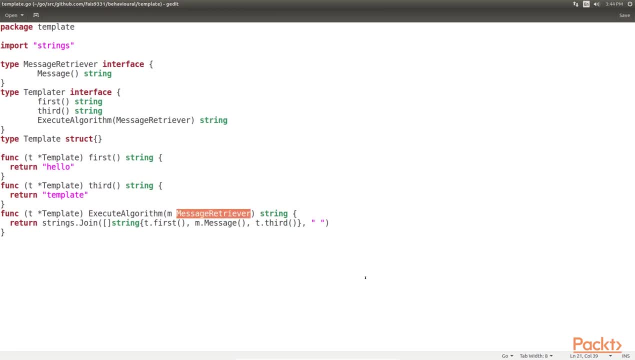 method that accepts the message retriever interface as an argument and returns the full algorithm: a single string done by joining the strings returned by the first message string and third methods. the strings dot join function has this signature: it takes an array of strings and joins them, placing the 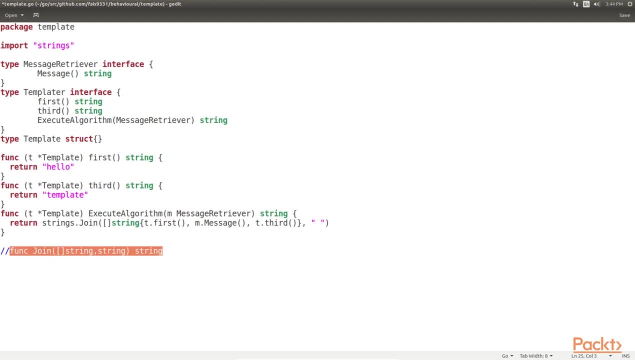 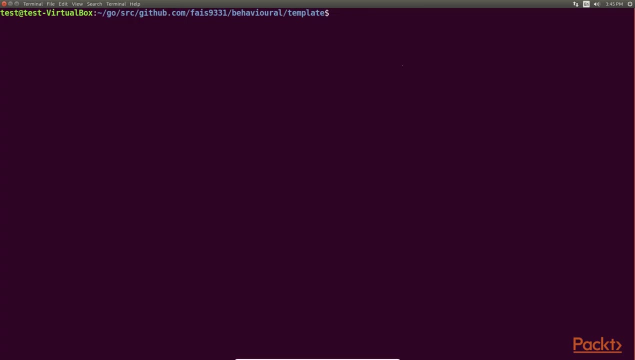 second argument between each item in the array. in our case, we create a string array on the fly to pass it as the first argument. then we pass a white space as the second argument. with this implementation, the tests must be passing already. let's save the file, navigate to the terminal and run the test. go, test. 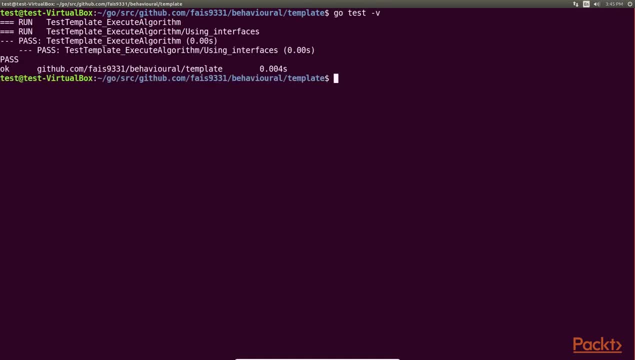 hyphen V: enter the tests passed. the test has checked that the string world is present in the returned result, which is the hello world template message. the hello text was the string returned by the first method. the world string was returned by our message retriever implementation and template was 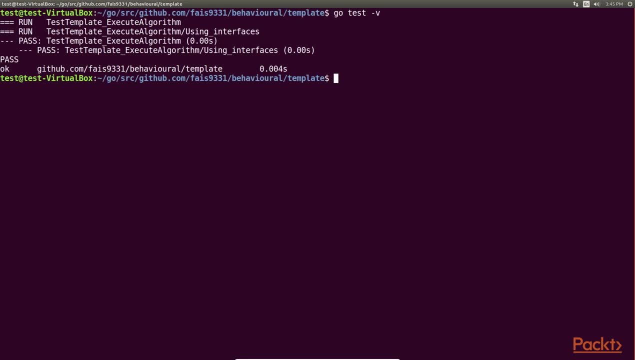 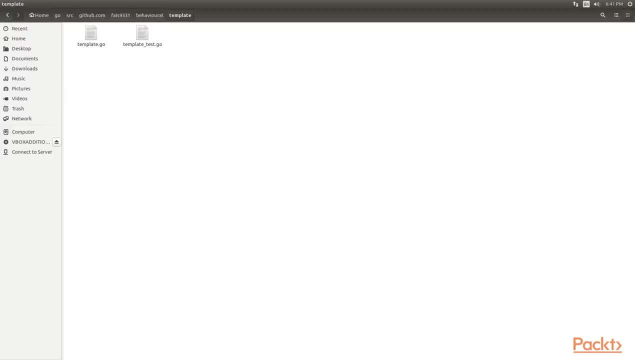 the string returned. by the third method. the white spaces are inserted by goes strings, dot join function. but any use of the template implementation dot execute algorithm type will always return hello something template in its result. this is not the only way to achieve the templates design pattern. we. 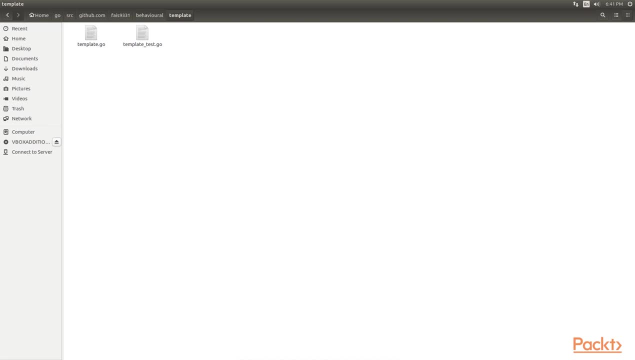 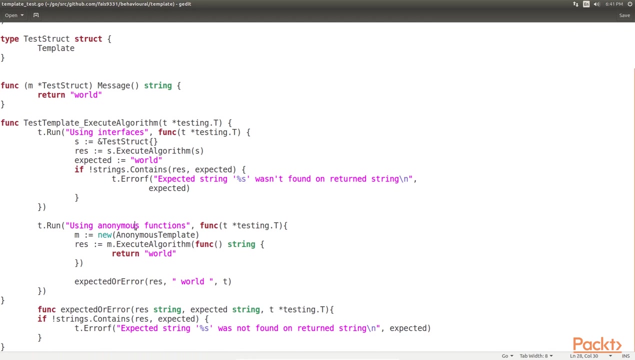 can also use an anonymous function to give our implementation the execute algorithm method. let's write a test in the same method that was used previously. so open the templates test dot, go file and add the code at the bottom of the file. our new test is called using anonymous functions. we have also 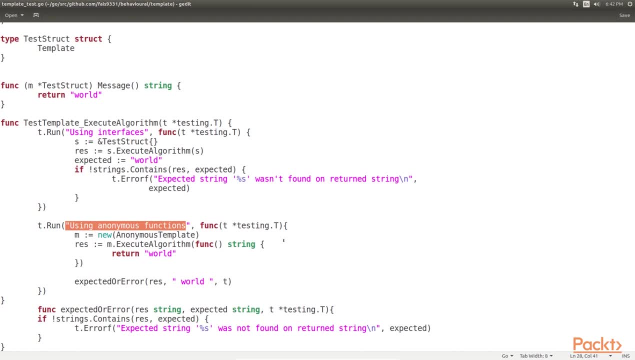 extracted the checking on the test to an external function to reuse it in this test. we have called this function expected or error, because it will fail with an error if the expected value isn't received. in our test we will create a type called anonymous template that replaces the previous template type, the 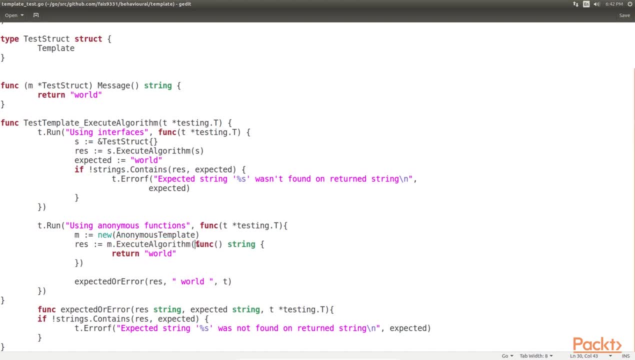 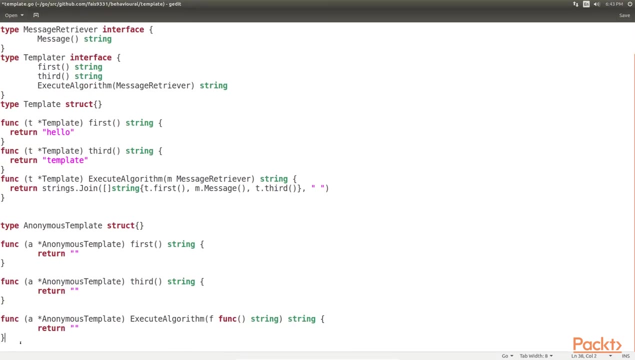 execute algorithm method of this new type accepts the funk method string type that we can implement directly in the test to return the string world. now let's save the file and move to the template dot go file. here we add the anonymous template type structure. the only difference with the template type is: 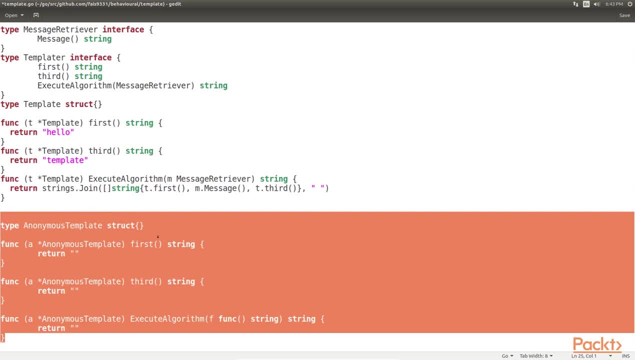 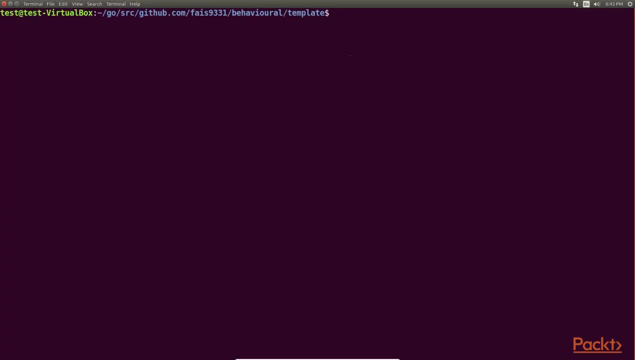 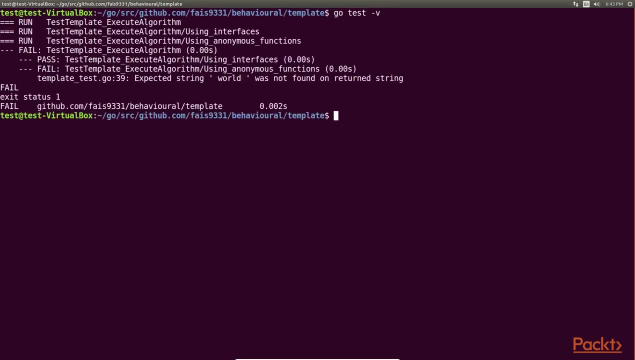 that the execute algorithm method accepts a function that returns a string instead of a message retriever interface. let's run the new test, save the file and go back to the terminal. let's run the test command, go test hyphen be. as you can read in the output of the test execution, the error is thrown on the using. 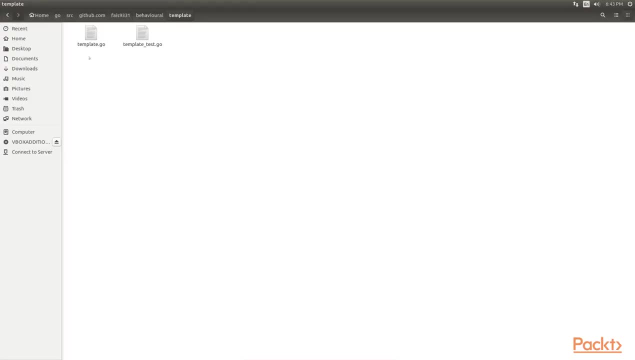 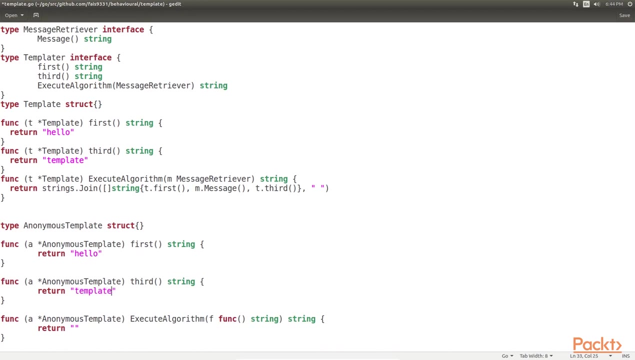 anonymous function test, which is what we were expecting. now, open the template dot go. let's write the implementation by modifying the return statements in the anonymous template type. the implementation is quite similar to the one in the template type. however, now we have passed a function called F that we 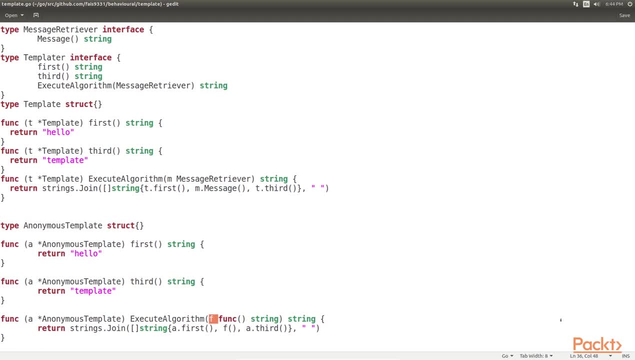 will use the second item in the string array we used on join function, as F is simply a function that returns a string. the only thing we need to do with it is to execute the proper place, which is the second position in the array. don't forget to save the file for the next test. 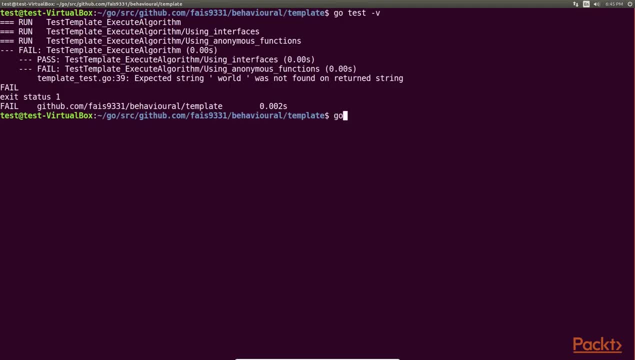 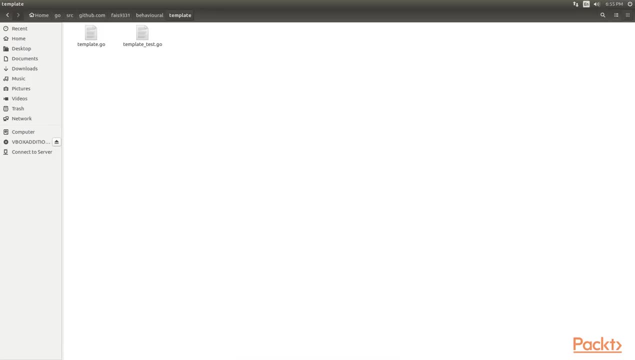 the terminal and run the tests again. awesome, now we know two ways to implement the template design pattern. now a question which may arise here is that how do you avoid the modifications on the interface? the problem of the previous approach, the now we have two templates to maintain, and we could end. 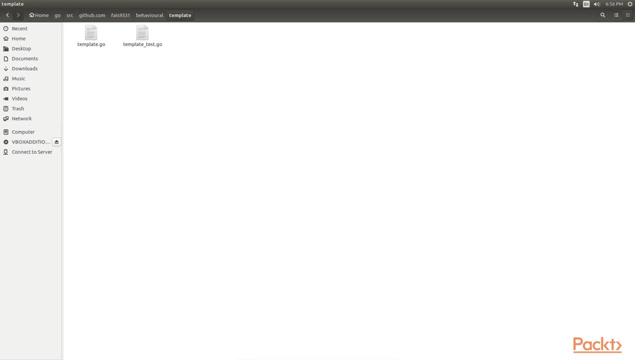 up duplicating. what can we do in the situation that we cannot change the interface we are using? our was the message receiver, but we want to use an anonymous function. now, Well, do you remember the adapter design pattern? We just have to create an adapter type that accepting a function string type. 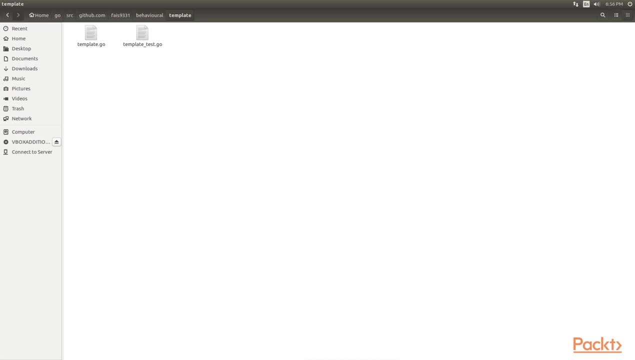 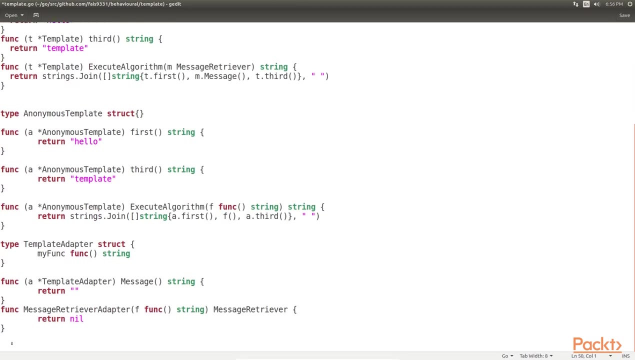 returns an implementation of the message receiver interface. We will call this type templateAdapter. Let's open templatego and add the templateAdapter. As you can see, the templateAdapter type has a field called myFunk, which is of the type FunkString. 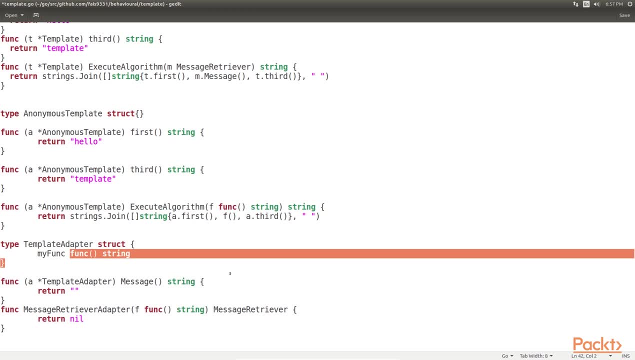 We have also defined adapter as private because it shouldn't be used without a function defined in the myFunk field. We have created a public function called the messageRetrieverAdapter. to achieve this. Let's save the file and go back to the template testgo. 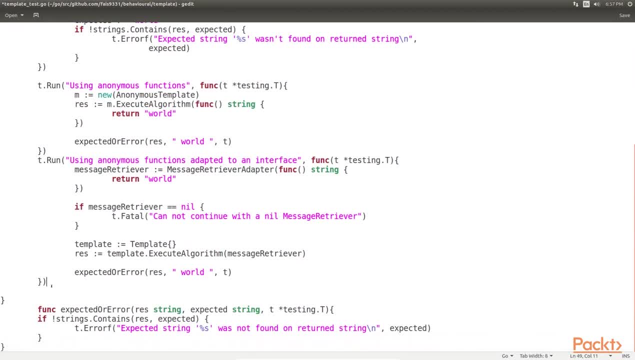 And here let's add the test. So this is how our test should more or less look like. Look at the statement where we called the messageRetrieverAdapter method. We passed an anonymous function as an argument defined as FunkString. Then we reused the previously defined template type from our first test. 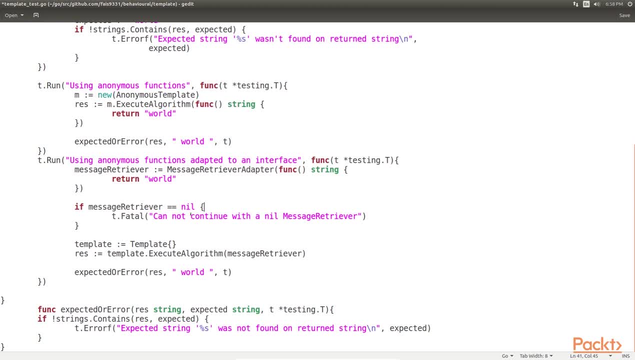 to pass the messageRetriever variable. Finally, we checked again with the expected or error method. Take a look at the messageRetrieverAdapter method. It will return a function that has nil value If strictly following the test-driven development rules. 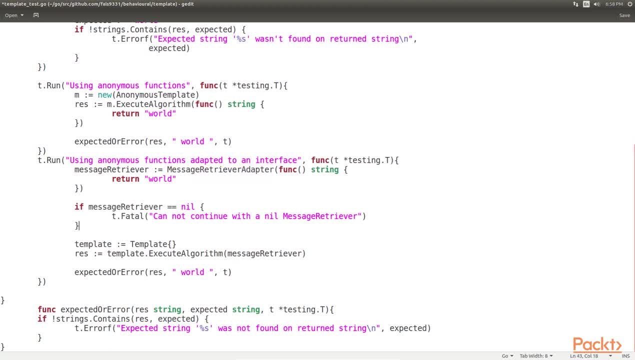 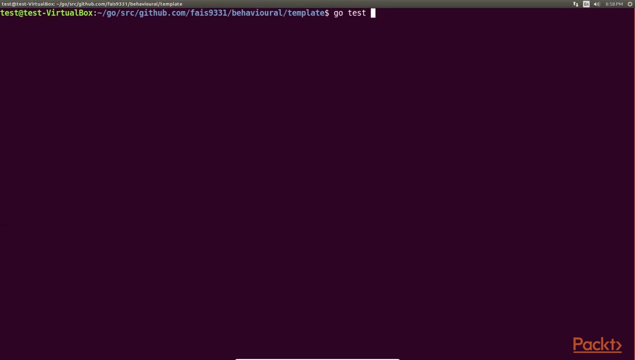 we must do tests first and they must not pass before implementation. That's why we returned nil on the messageRetrieverAdapter function. So let's run the tests First. save the file and move to the terminal. Run the command: go test-v. 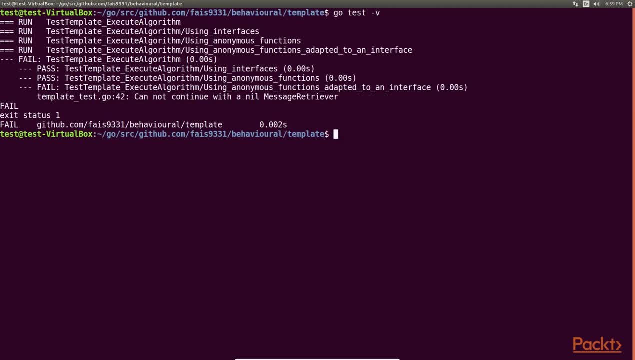 The test fails on line 42 of the code and it doesn't continue Again. depending on how you wrote your code, the line representing your error could be somewhere else. We stop test execution because we will need a valid message receiver interface when we call the executeAlgorithm method. 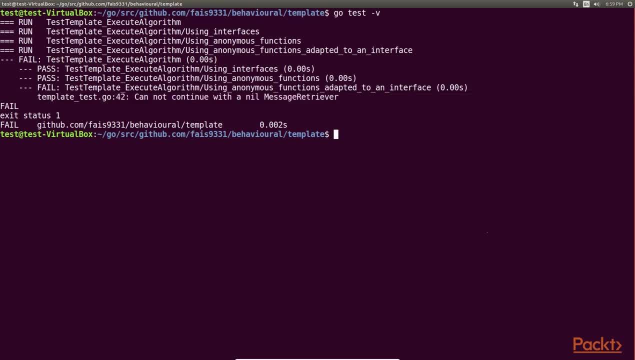 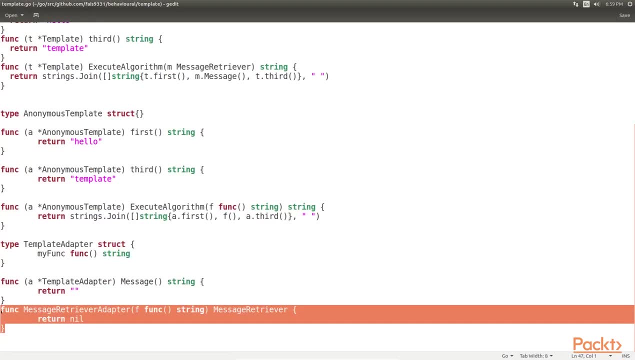 For the implementation of the adapter for our template pattern. we will start with messageRetrieverAdapter method. So let's go back to the templatego, Let's modify the messageRetrieverAdapter. It's very easy, right? You could be wondering what happens if we pass nil value for the f argument. 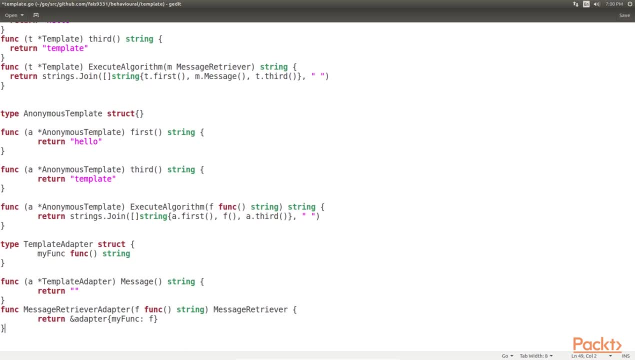 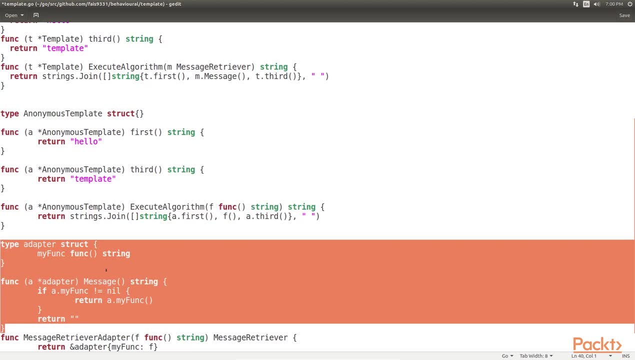 Well, we will cover this issue by calling the myFunk function. Now let's modify the type templateAdapter struct, So the adapter type is finished with this implementation. When calling the message function, we check that we actually have something stored in the myFunk function before calling. 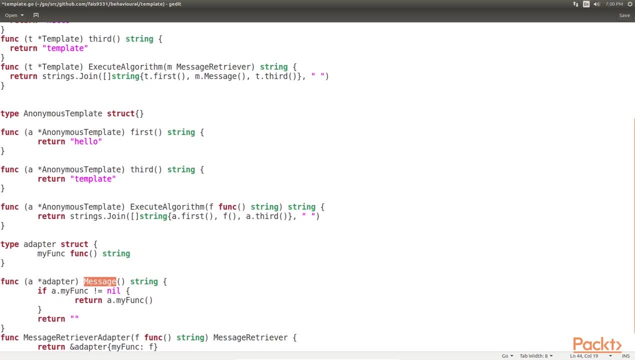 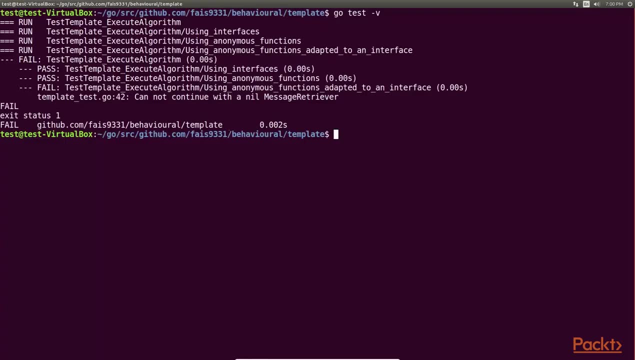 If nothing was stored, we return an empty string. Now our third implementation of the template type, using the adapter pattern, is done. Save the file and move to the terminal. Let's run the test command. As you can see, we have passed the test- Wonderful. 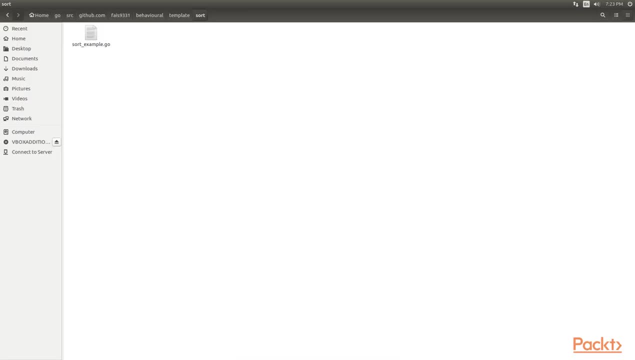 Now let's see how to look for the template pattern in Go's source code. The sort package in Go's source code can be considered a template implementation of a sort algorithm As defined in the package itself. the sort package provides primitives for sorting slices and user-defined collections. 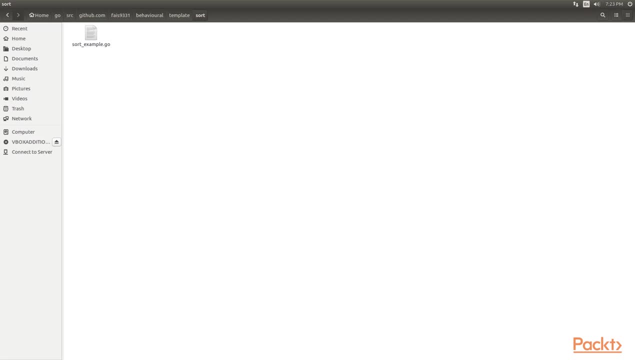 Here we can also find a good example of why Go authors aren't worried about implementing generics. Sorting the lists is maybe the best example of generic uses in other languages. The way that Go deals with this is very elegant too. It deals with this issue with an interface. 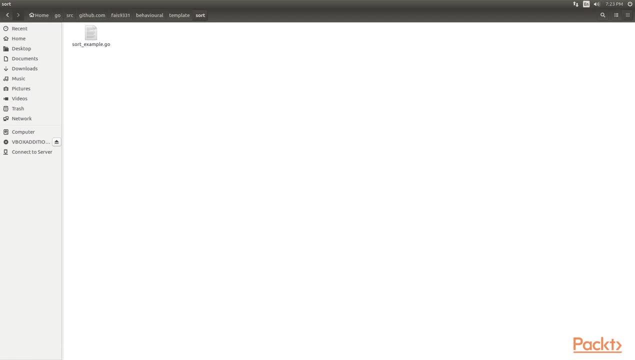 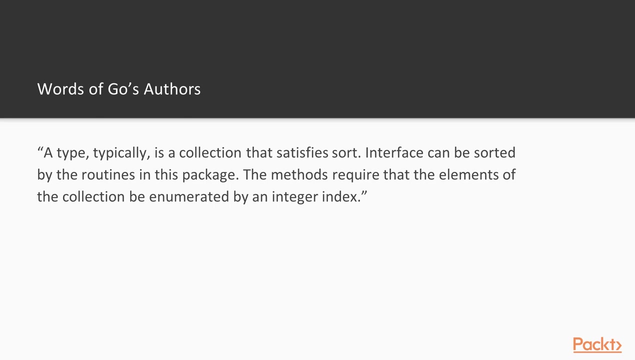 Let me show you this interface. I have already created the file sort__examplego. Let me open this. This is the interface for lists that need to be sorted by using the sort package. In the words of Go's authors, a type typically is a collection that satisfies sort. 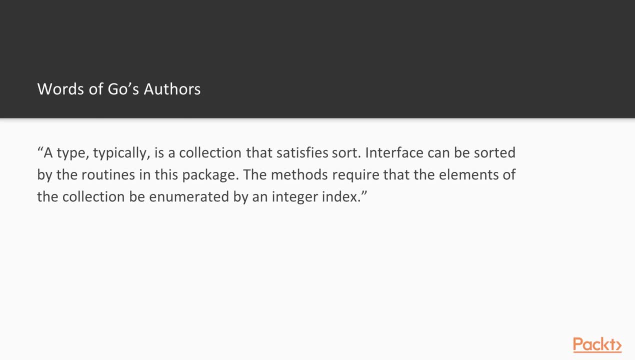 Interface can be sorted by the routines in this package. The methods require the list to be sorted. Let the elements of the collection be enumerated by an integer index. In other words, write a type that implements this interface so that the sort package can be used to sort any slice. 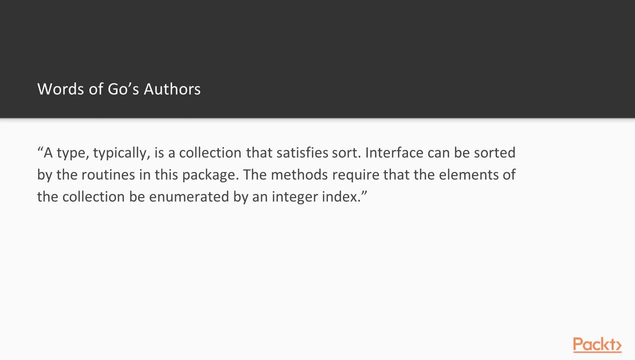 The sorting algorithm is the template, and we must define how to retrieve values in our slice. If we peek in the sort package, we can also find an example of how to use the sorting template, but we will create our own example Here. add the lines of code, as I do. 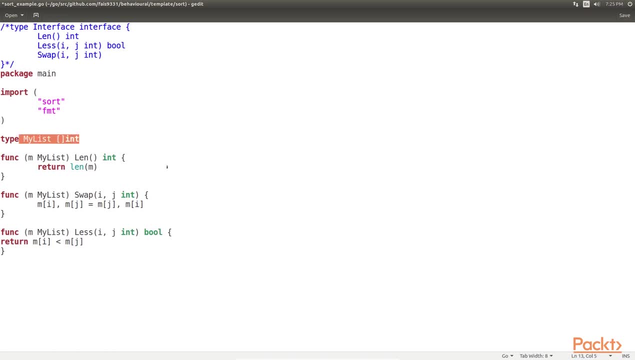 First we have done a very simple type that stores an int list. This could be any kind of list, usually a list of some kind of struct. Then we have implemented the sortinterface interface by defining the len swap and less methods. 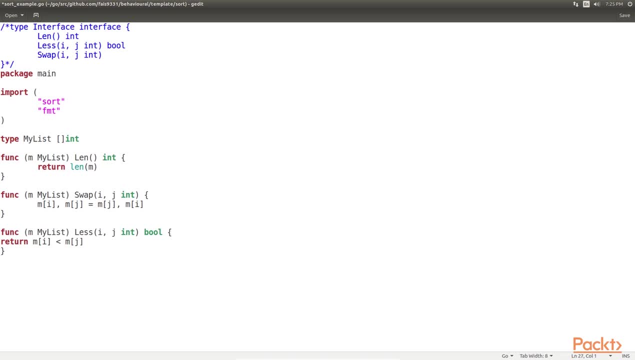 Finally, let's write the main function. The main function creates an unordered list of numbers of the myList type. We print the list that we created unordered and then we sort it. The sortsort method actually modifies our variable instead of returning a new list. 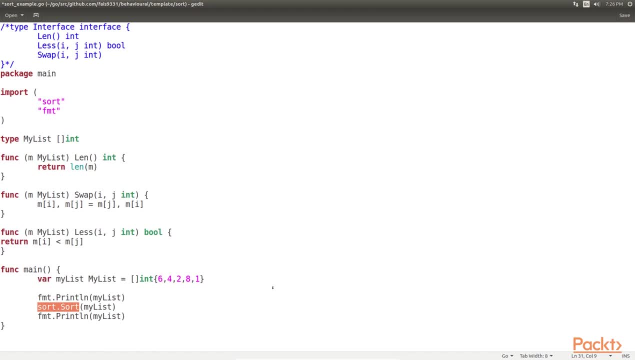 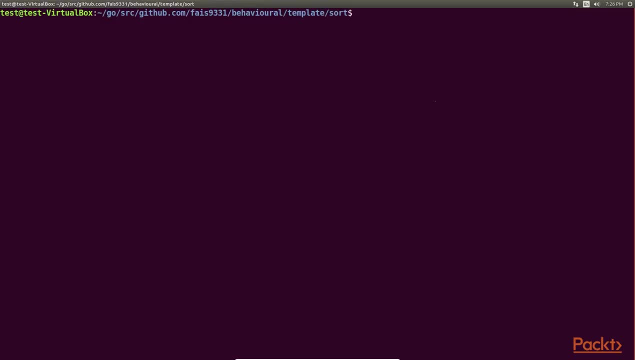 so beware. Finally, we print again the resulting list. Now we are ready to see the console output of this main method. Save the file and open the terminal. Run the command. gorunsortexamplego, The sortsort function has sorted our list in a transparent way. 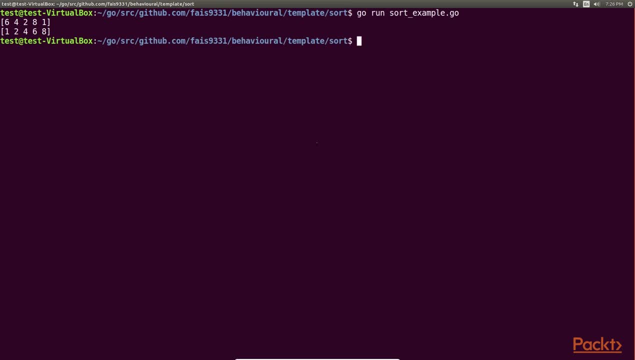 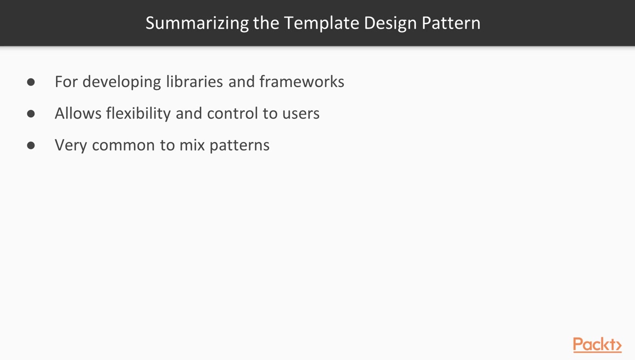 It has a lot of code written and delegates len, swap and less methods to an interface, like we did in our template delegating to the message retriever interface, Superb. Now let me summarize the template design pattern. So we wanted to put a lot of focus on this pattern. 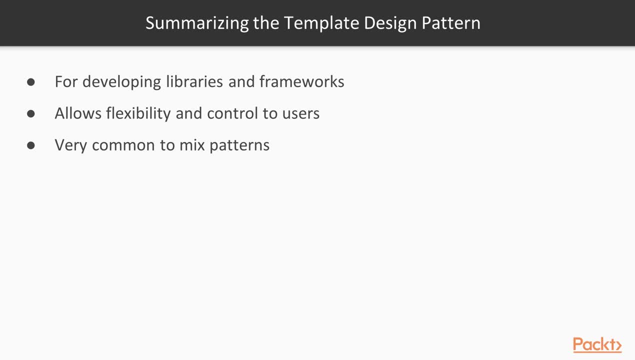 because it is very important when developing libraries and frameworks and allows a lot of flexibility and control to users of our library. We have also seen again that it's very common to mix patterns to provide flexibility to the users, Not only in a behavioral way.